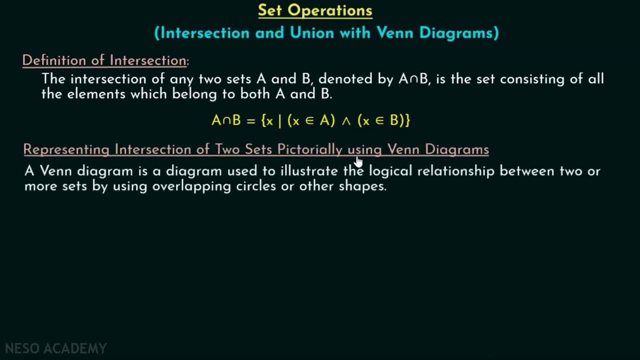 Now let's see how to represent intersection of two sets pictorially using Venn diagrams. A Venn diagram is a diagram used to illustrate the logical relationship between two or more sets. by using overlapping sets, This diagram is a way to illustrate the logical relationship between two or more sets. 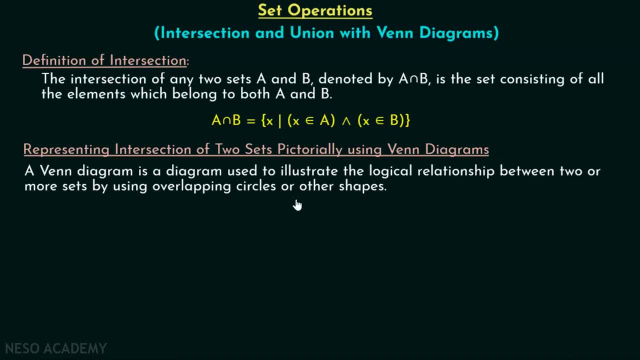 And we can do this by using overlapping circles or other shapes. First we will have some basic understanding about this. Then we will move on to how to represent an intersection using Venn diagrams. Here is the basic overview. A set is usually represented by a circle and the elements of the set lies within the circle. 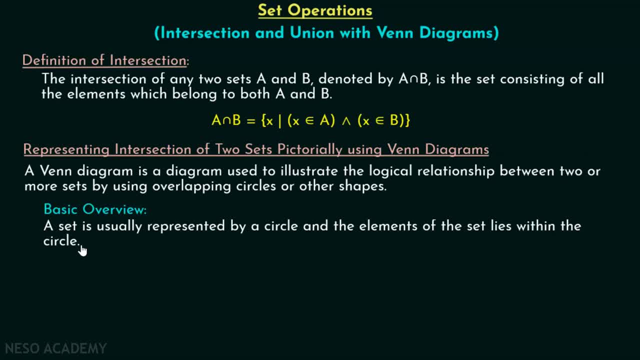 So if we want to represent a set, then we can represent it by a circle And the elements of that set lies within that circle. A universal set or universe of discourse is represented by a rectangle. Every element under consideration lies within the rectangle. 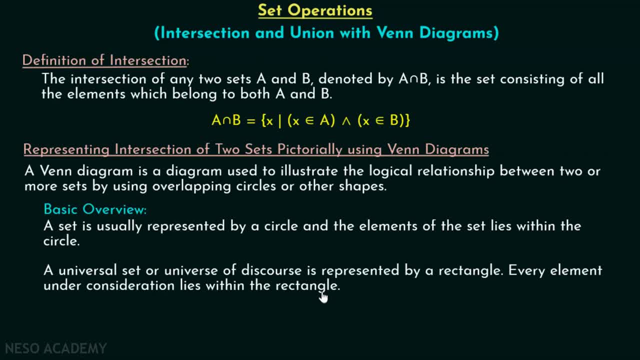 So we have two things. One is circle and the other one is rectangle. Rectangle usually represents a universal set. Here every element under consideration lies within the rectangle, And we usually represent sets by circles. So here is one example. This is how a vector 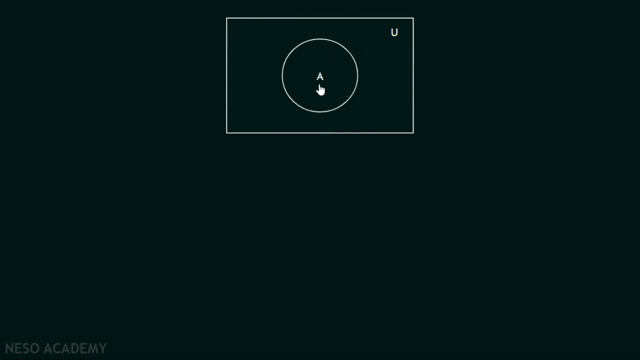 This is how a Venn diagram looks like. Here we have a circle- This is set A, which is represented by a circle, And we have this rectangle outside this circle, which is universe of discourse or universal set. So here I am, representing universe of discourse or universal, set by capital U. 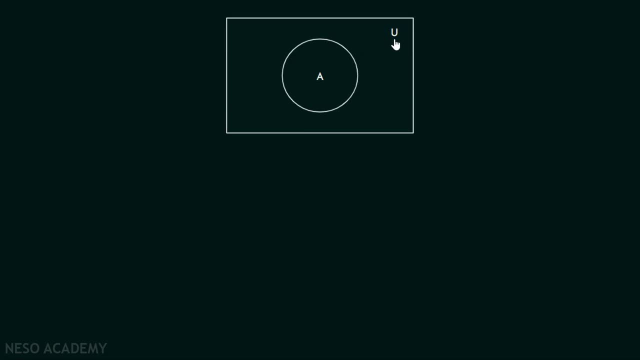 We can also use capital E to represent universe of discourse, But that's not a problem, It's just a notation. You can use any one of them Here. this circle is representing set A And this rectangle is representing set B And this rectangle is representing universal set. 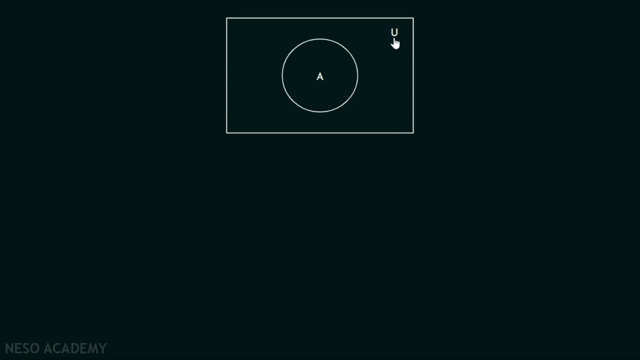 Now let's see the pictorial representation of intersection of sets A and B. This is how it looks like. Here we have two sets, A and B, And you can see over here that these two circles are overlapping. They are not separate, They are overlapping. 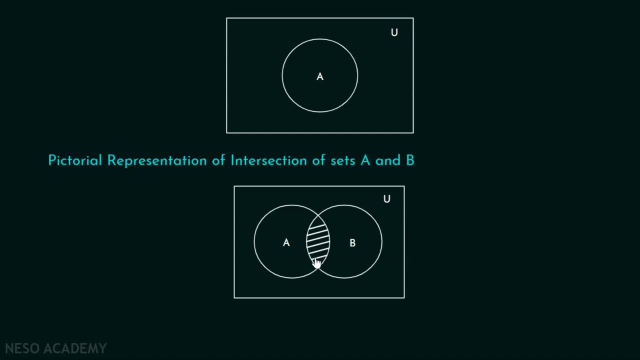 This means there are some elements which are common in between them. Here the shaded region is the common area between A and B, That is, A intersection B. This is the common area I was talking about. Here we have all the common elements between A and B. 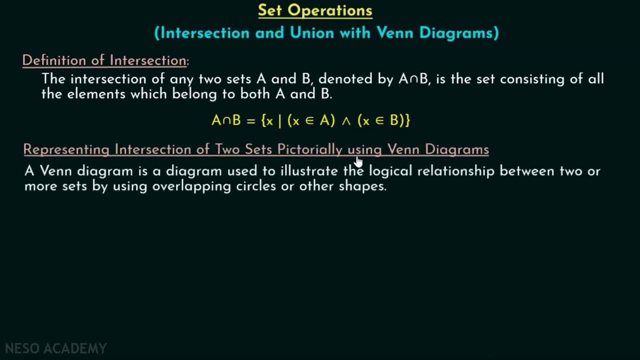 Now let's see how to represent intersection of two sets pictorially using Venn diagrams. A Venn diagram is a diagram used to illustrate the logical relationship between two or more sets. by using overlapping sets, This diagram is a way to illustrate the logical relationship between two or more sets. 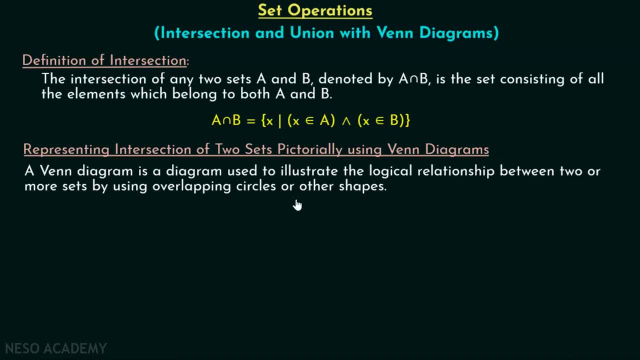 And we can do this by using overlapping circles or other shapes. First we will have some basic understanding about this. Then we will move on to how to represent an intersection using Venn diagrams. Here is the basic overview. A set is usually represented by a circle and the elements of the set lies within the circle. 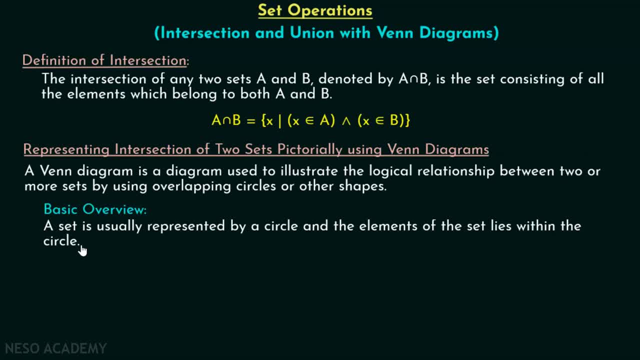 So if we want to represent a set, then we can represent it by a circle And the elements of that set lies within that circle. A universal set or universe of discourse is represented by a rectangle. Every element under consideration lies within the rectangle. 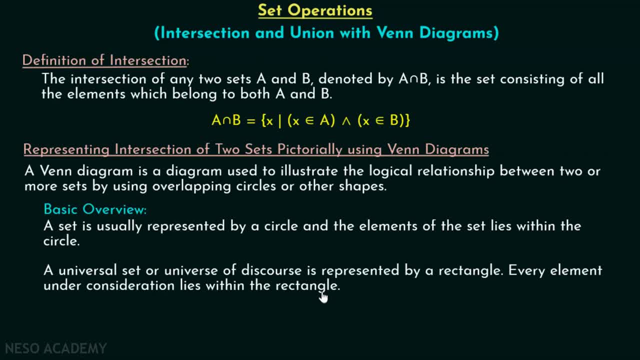 So we have two things. One is circle and the other one is rectangle. Rectangle usually represents a universal set. Here every element under consideration lies within the rectangle, And we usually represent sets by circles. So here is one example. This is how a vector 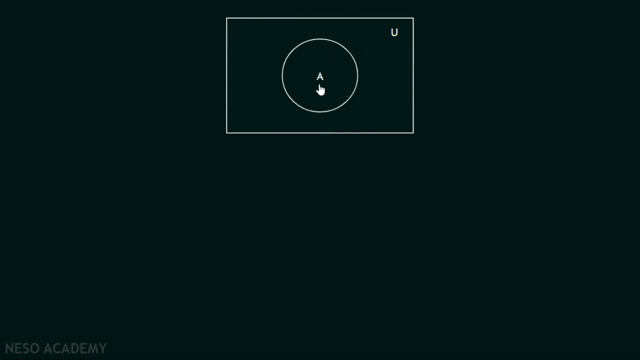 This is how a Venn diagram looks like. Here we have a circle- This is set A, which is represented by a circle, And we have this rectangle outside this circle, which is universe of discourse or universal set. So here I am, representing universe of discourse or universal, set by capital U. 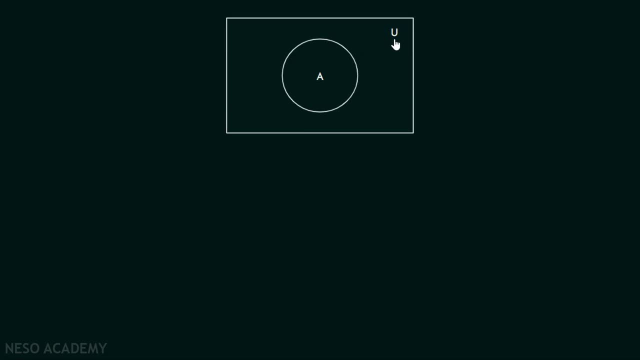 We can also use capital E to represent universe of discourse, But that's not a problem, It's just a notation. You can use any one of them Here. this circle is representing set A And this rectangle is representing set B And this rectangle is representing universal set. 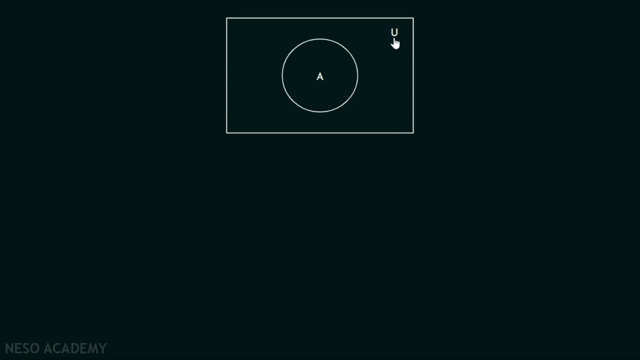 Now let's see the pictorial representation of intersection of sets A and B. This is how it looks like. Here we have two sets, A and B, And you can see over here that these two circles are overlapping. They are not separate, They are overlapping. 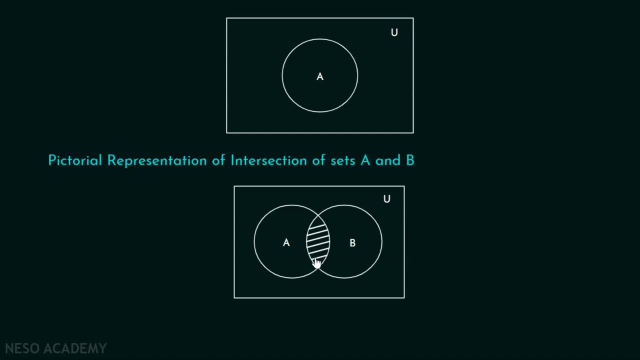 This means there are some elements which are common in between them. Here the shaded region is the common area between A and B, That is, A intersection B. This is the common area I was talking about. Here we have all the common elements between A and B. 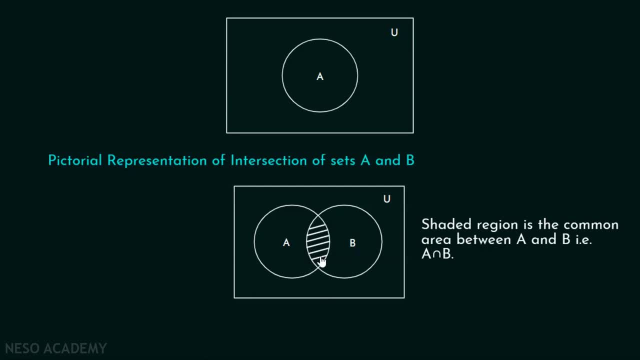 So this overlapping area is called the common area, Or in other words we can say: this is A intersection B. Here this area represents only A and not B, And here this area represents only B and not A. But this area is common area between A and B. 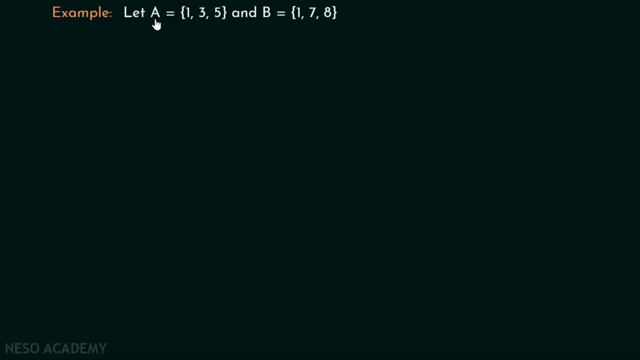 That is A intersection B. Now let's see one example: Let A is this set and B is representing this set. Okay, We can represent these two sets by a Venn diagram. Here you can see that I am using two circles to represent set A and set B. 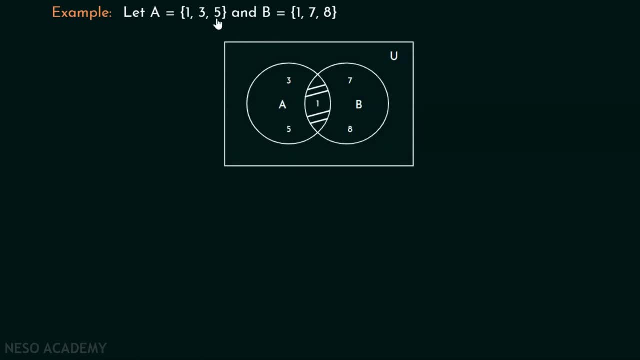 Here, within this set A, we have elements 1,, 3 and 5. And in set B we have 1,, 7, 8. We can clearly see that 1 is common element between A and B, So I am putting this over here. 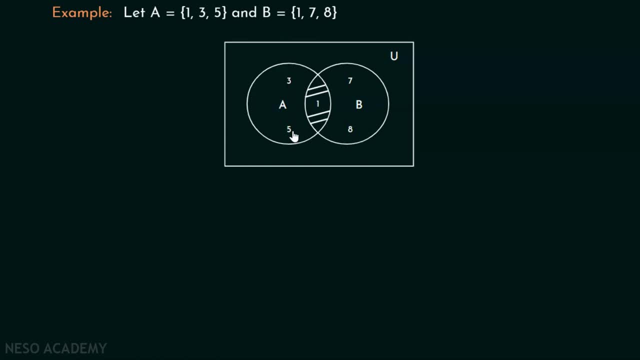 That is, in this common area. Right Here we have elements 3 and 5, which are only in A and not in B, And here we have 7 and 8, which are in B and not in A. Now let's discuss the definition of union. 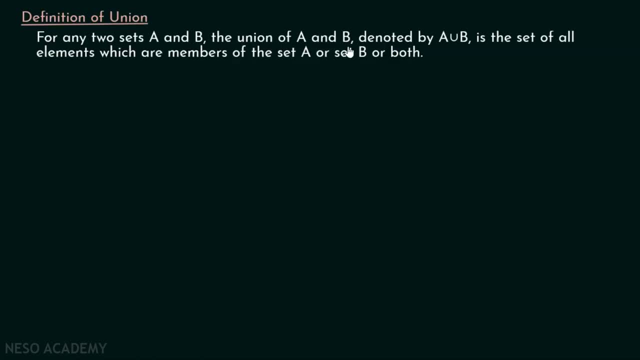 For any two sets, A and B. the union of A and B denoted by this particular symbol- this is union symbol- is the set of all elements which are members of the set A or set B, or both. That is, A union. B is equal to. 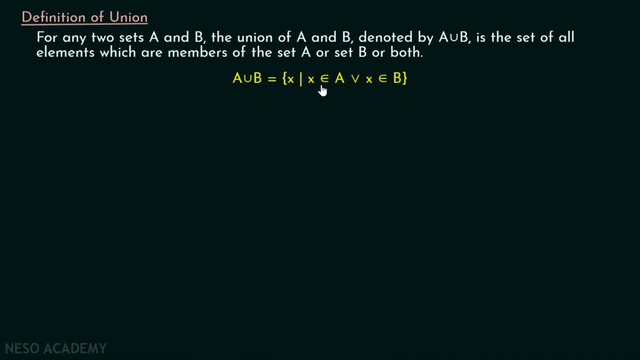 set of all x, such that x belongs to A or x belongs to B. In case of intersection, we have AND over here, In case of union, we have OR. This is a common diagram of union of sets. This is how it looks like. 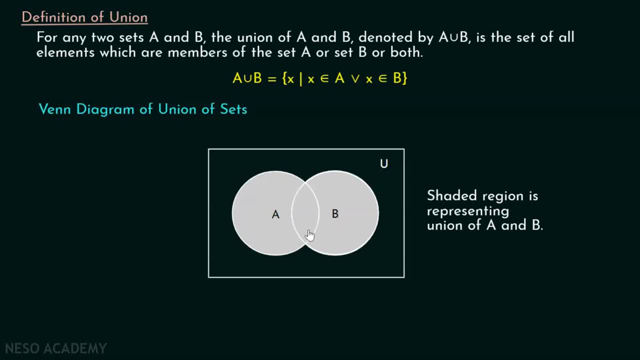 Here it is clear that set A is represented by this circle and set B is represented by this circle. Union of A and B is nothing but either A or B or both. That means everything under consideration. This shaded region is representing union of A and B. 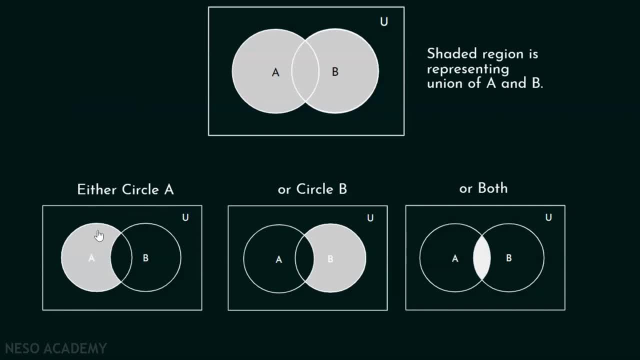 In other words, we can say that either circle A- this is only circle A and not B, This is only circle B and not A, But this portion represents both A and B. So union means either A or B or both. That means everything. 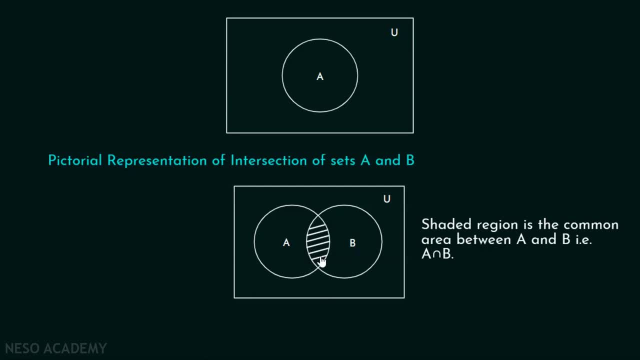 So this overlapping area is called the common area, Or in other words we can say: this is A intersection B. Here this area represents only A and not B, And here this area represents only B and not A. But this area is common area between A and B. 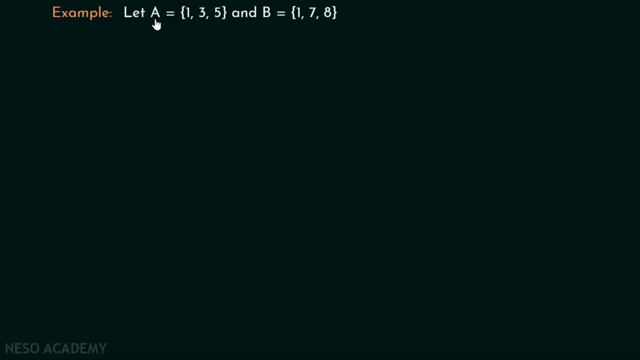 That is A intersection B. Now let's see one example: Let A is this set and B is representing this set. Okay, We can represent these two sets by a Venn diagram. Here you can see that I am using two circles to represent set A and set B. 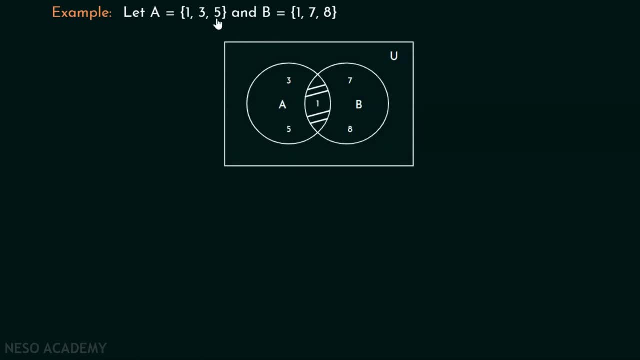 Here, within this set A, we have elements 1,, 3 and 5. And in set B we have 1,, 7, 8. We can clearly see that 1 is common element between A and B, So I am putting this over here. 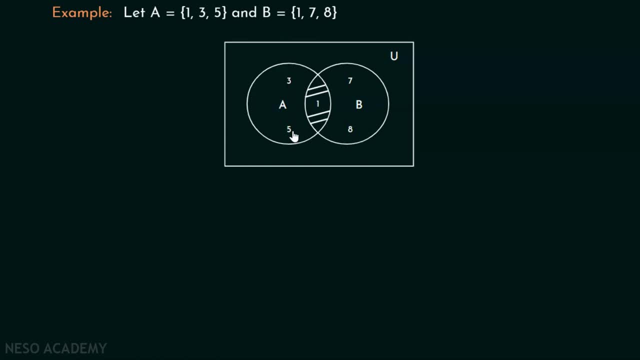 That is, in this common area. Right Here we have elements 3 and 5, which are only in A and not in B, And here we have 7 and 8, which are in B and not in A. Now let's discuss the definition of union. 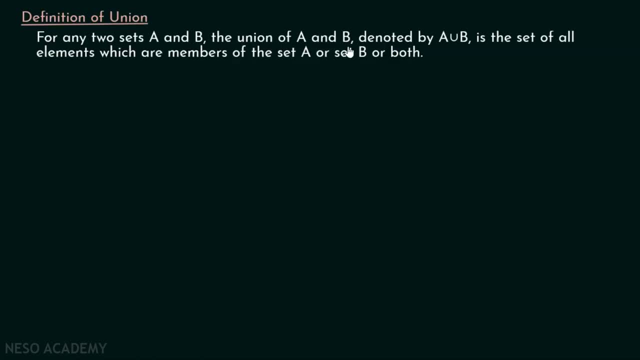 For any two sets, A and B. the union of A and B denoted by this particular symbol- this is union symbol- is the set of all elements which are members of the set A or set B, or both. That is, A union. B is equal to. 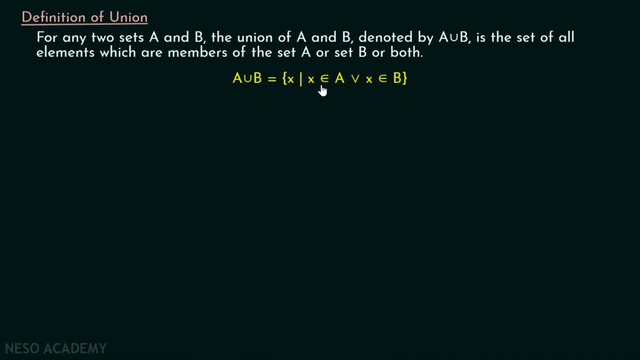 set of all x, such that x belongs to A or x belongs to B. In case of intersection, we have AND over here, In case of union, we have OR. This is a common diagram of union of sets. This is how it looks like. 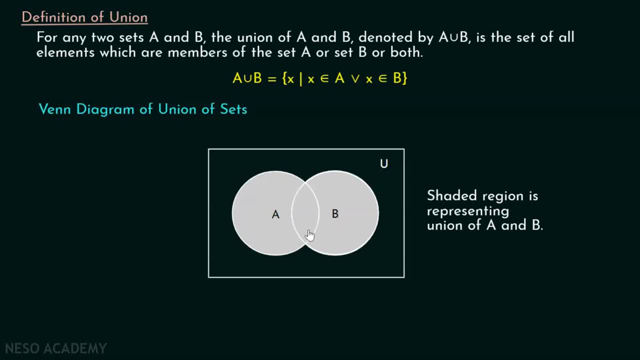 Here it is clear that set A is represented by this circle and set B is represented by this circle. Union of A and B is nothing but either A or B or both. That means everything under consideration. This shaded region is representing union of A and B. 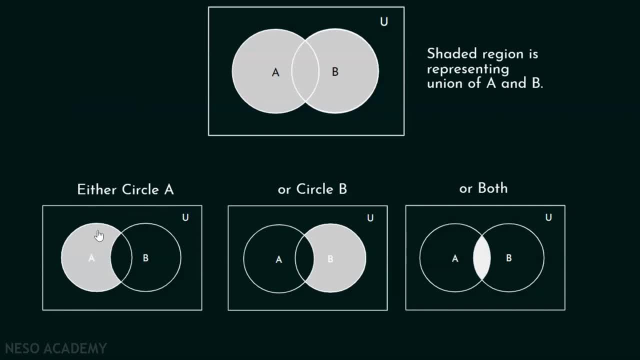 In other words, we can say that either circle A- this is only circle A and not B, This is only circle B and not A, But this portion represents both A and B. So union means either A or B or both. That means everything.